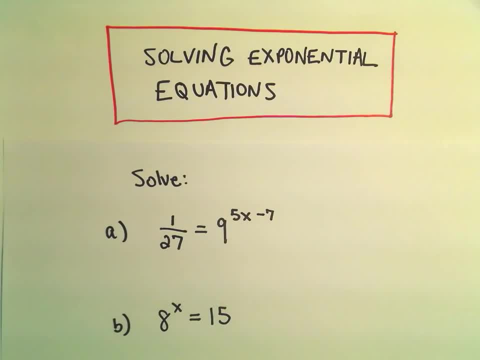 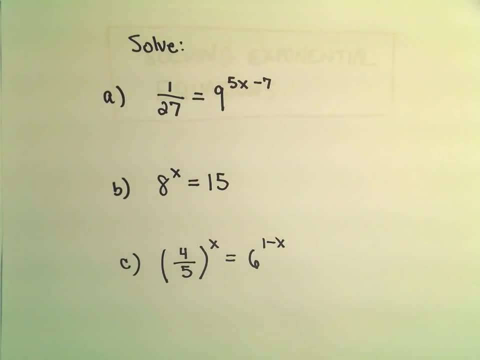 Alright, in this video I'm going to do a few examples of solving exponential equations, And three examples here. On the first one, we're not going to have to. We can just kind of use a little clever trick, I think, to get our value exactly. 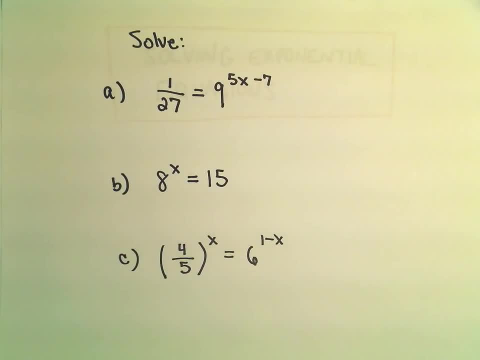 To get our exact values in part B and C, though, we're going to have to use some logarithms. But for part A, here we've got 1 over 27 equals 9 raised to the 5x minus 7.. 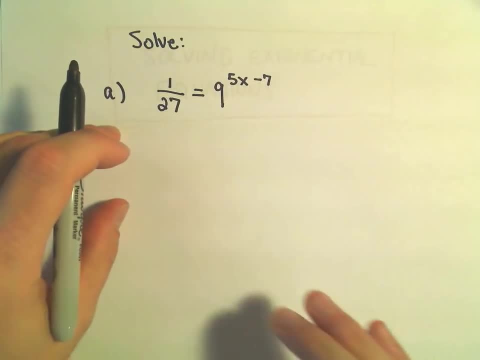 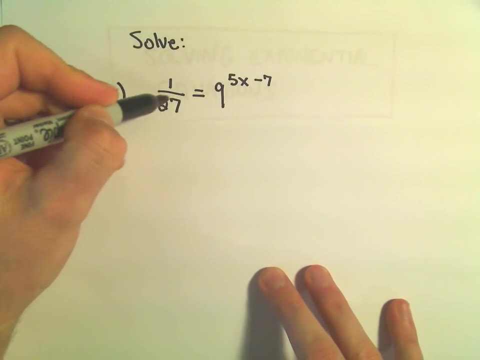 And the thing that sticks out to me in this problem is that 27 is a power of 3.. And I know it's 1 over 27,, but in the denominator, 27 is a power of 3.. 9 is also a power of 3, so I'm going to rewrite 27 as 3 cubed. 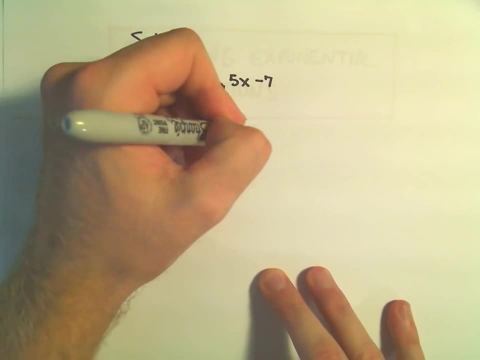 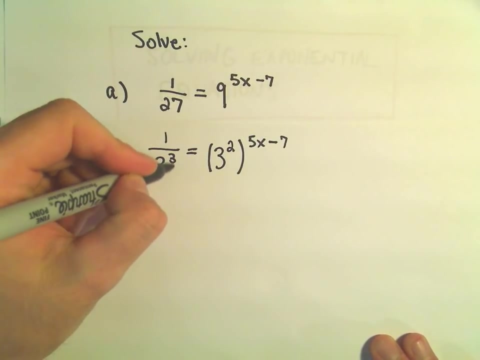 9, we can write that as 3 squared And then we still have our 5x minus 7.. Well, on the left side, I'm going to bring my denominator, We're going to bring our denominator upstairs by writing it as 3 to the negative 3rd. 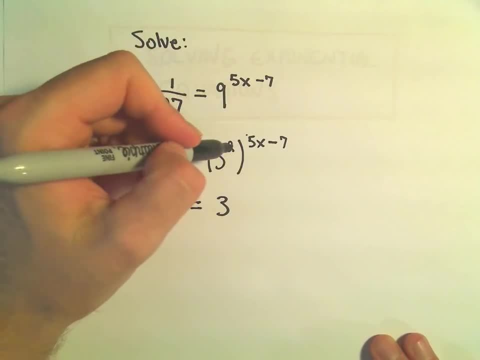 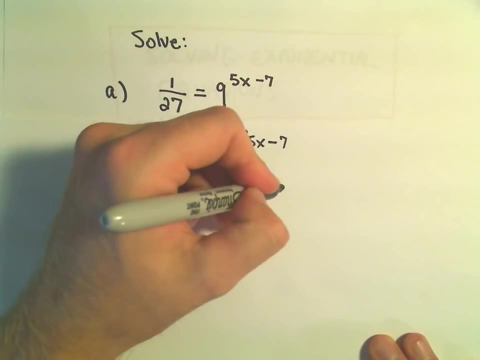 And then on the right side again, since these are in parentheses, we multiply. So 2 times 5x would be 10x. 2 times negative 7 would be negative 14.. And now, since we have like bases, we can just set the exponents equal to each other and solve. 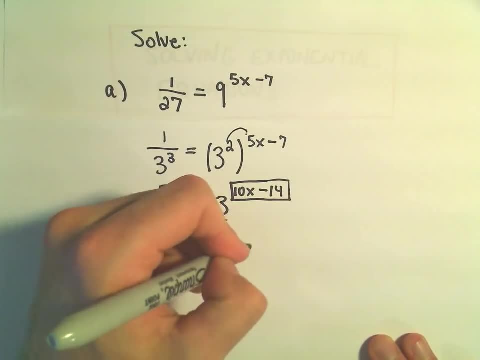 So we would get negative 3 equals 10x minus 14.. Well, I can add 14 to both sides. That would give me 11 on the left side and just 10x on the right side, And now I can simply just divide both sides by 10.. 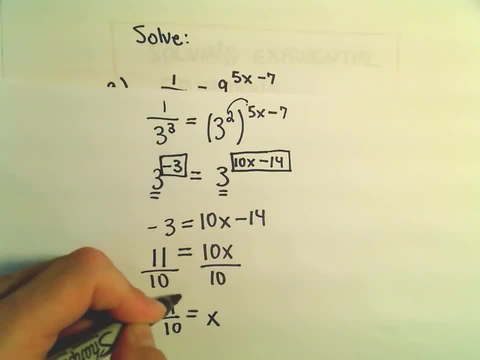 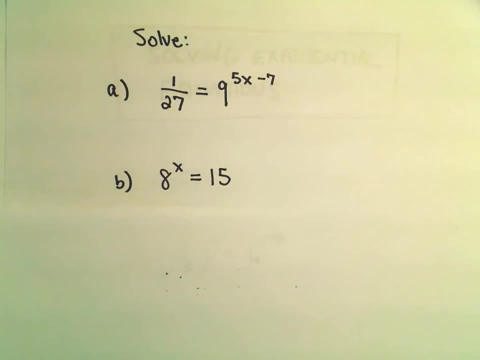 And it says: my solution would be: x equals 11 over 10.. Okay, so nothing too bad there. However, if you look at the second example, 8x equals 15, well, you know, I don't know how to write these with an equivalent sort of base, like we did in the last example. 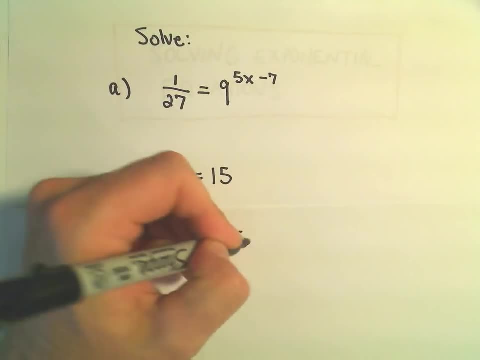 So what we do at this point is the trick to get you know: eventually I want to solve for x And I want to get the x away from being the exponent. And you know again, in general, this is an exponential function. 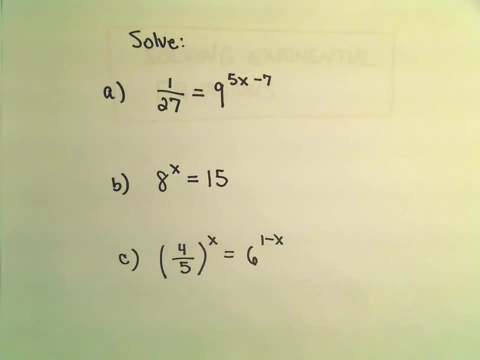 To get our exact values in part B and C, though, we're going to have to use some logarithms. But for part A, here we've got 1 over 27 equals 9 raised to the 5x minus 7.. 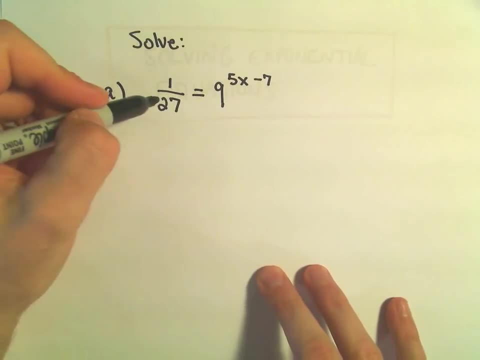 The thing that sticks out to me in this problem is that 27 is a power of 3.. And I know it's 1 over 27,, but in the denominator, 27 is a power of 3.. 9 is also a power of 3, so I'm going to rewrite 27 as 3 cubed. 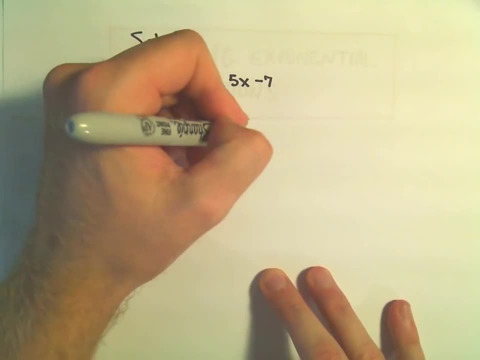 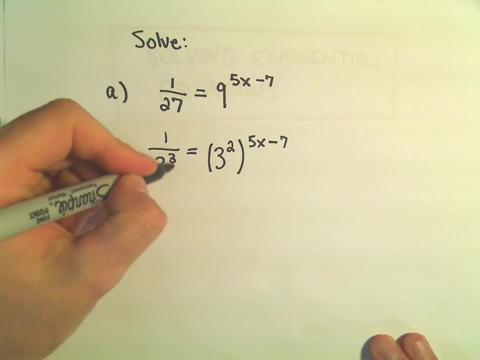 9, we can write that as 3 squared, and then we still have our 5x minus 7.. Well, on the left side, I'm going to bring my denominator upstairs by writing it as 3 to the 3.. 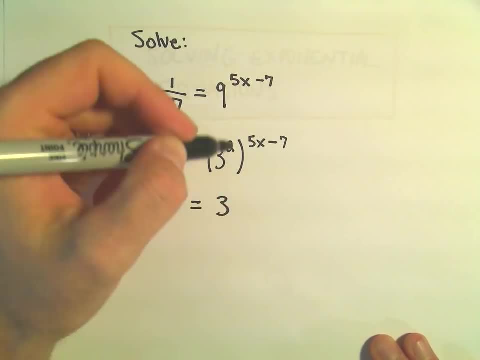 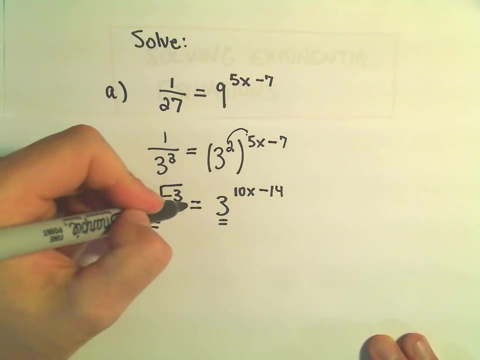 And then on the right side again, since these are in parentheses, we multiply. So 2 times 5x would be 10x. 2 times negative 7 would be negative 14.. And now, since we have like bases, we can just set the exponents equal to each other and solve. 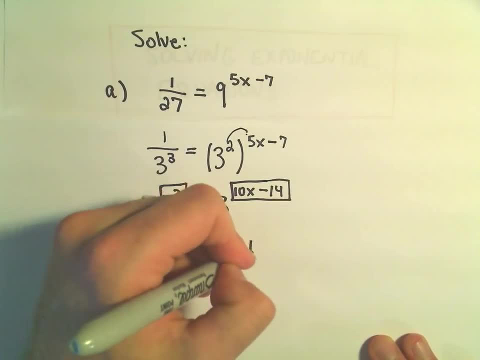 So we would get negative 3 equals 10x minus 14.. Well, I can add 14 to both sides. That would give me 11 on the left side And just 10x on the right side, And now I can simply just divide both sides by 10.. 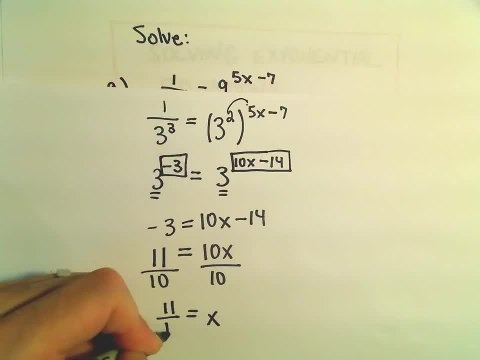 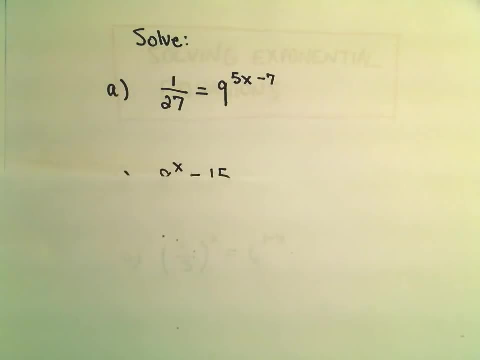 And it says: my solution would be: x equals 11 over 10.. Okay, so nothing too bad there. However, if you look at the second example, 8x equals 15, well, you know, I don't know how to write these with an equivalent sort of base, like we did in the last example. 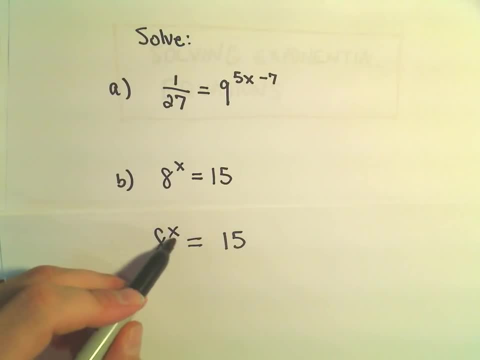 So what we do at this point is the trick to get you know: eventually I want to solve for x And I want to get the x away from being the exponent. And you know again, in general, this is an exponential function. 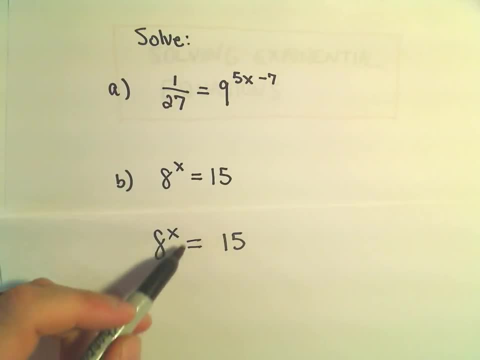 You always want to think about what's the inverse, what undoes something? And the inverse of an exponential is a logarithm. So I'm going to take a logarithm of both sides. You can use any logarithm you want. Most of the times we're going to use log base 10 or the natural logarithm so that we can put it in a calculator. 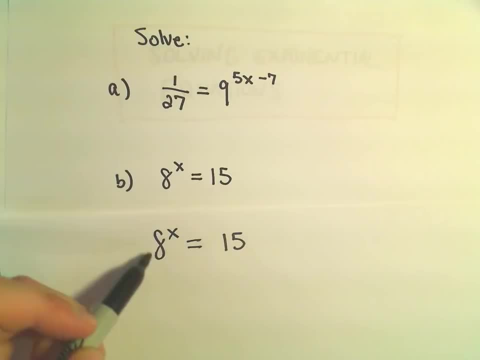 You always want to think about what's the inverse, what undoes something? And the inverse of an exponential is a logarithm. So I'm going to take a logarithm of both sides. You can use any logarithm you want. Most of the times we're going to use log base 10 or the natural logarithm. 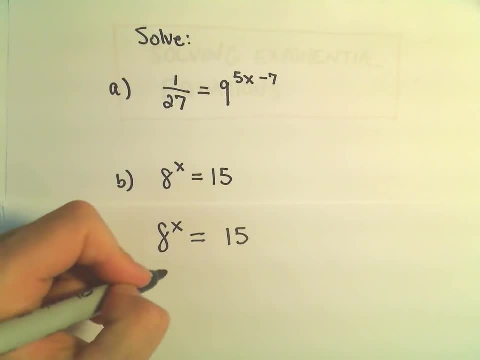 So I'm going to take a logarithm of both sides. So I'm going to take a logarithm of both sides So that we can put it in a calculator. So I'm just going to take the natural logarithm of the left side. 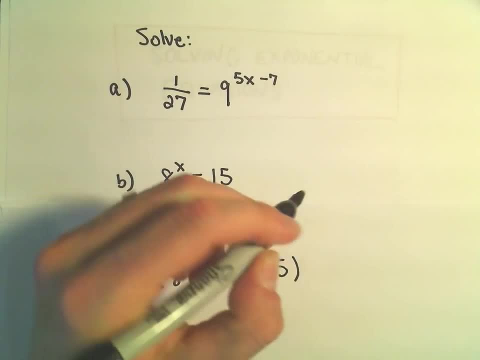 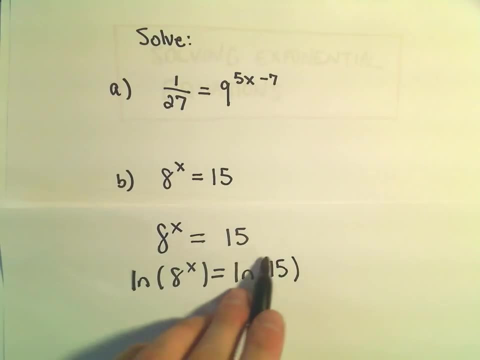 Well, hey, that means I have to take the natural logarithm of the right side as well. Okay, and don't get thrown off. You know the natural logarithm of 15, that's some number I always. you know I don't turn these into decimals because then you're approximating. 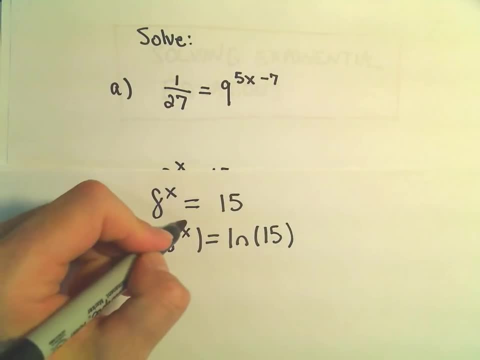 And I want to keep them exact. So remember this property that says: if you have exponents, you can bring them out front, And this is the whole point of using the logarithm in the first place. So on the left side we would have: x times the natural logarithm of 8 equals the natural logarithm of 15.. 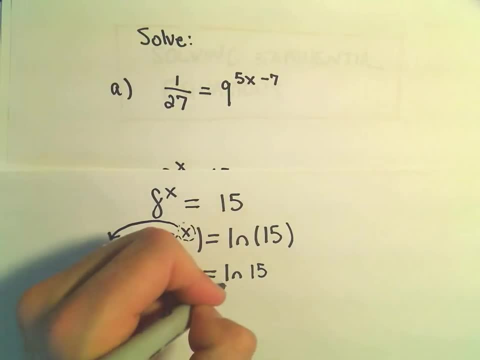 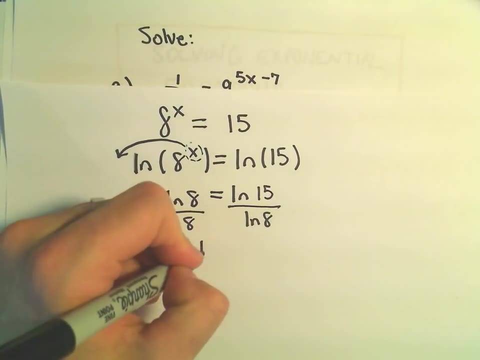 And well, if we want to solve for x, we can just simply divide both sides by that number, the natural logarithm of 8.. And on the right side we'll just have ln of 15 over ln of 8. And to me, hey, that's our solution. 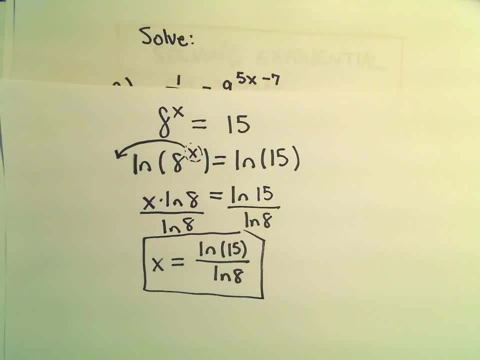 So again, you can always plug this into a calculator if you want a nice decimal approximation. But you know, I'm just going to leave it right there. It's exact, And hey, that's what we need. So one more example here. 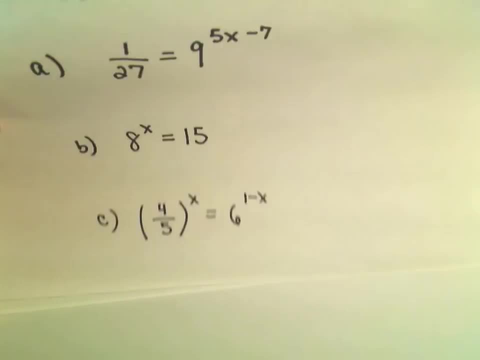 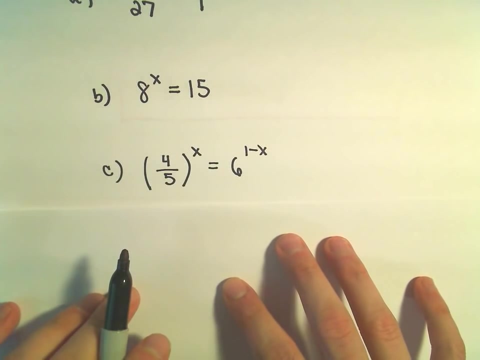 We've got 4 fifths raised to the x, equals 6 raised to the 1 minus x. Well, exact same thing, You know. I see variables upstairs as exponents. The way I'm going to get those away from being exponents is by throwing logarithms onto both sides. 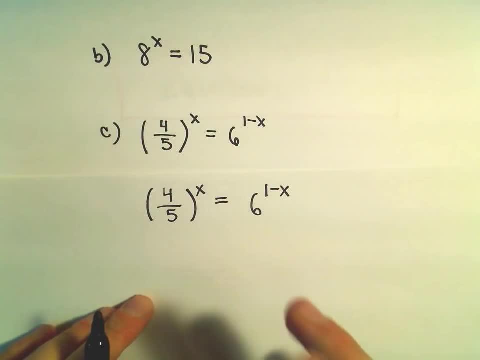 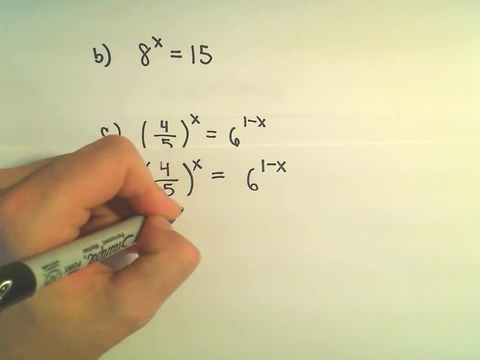 Again, you can use any type of logarithm you want. You obviously have to use the same one on each side. I'm just going to use the natural logarithm again. So we have the natural logarithm of 4 fifths raised to the x equals the natural logarithm of 6 raised to the 1 minus x. 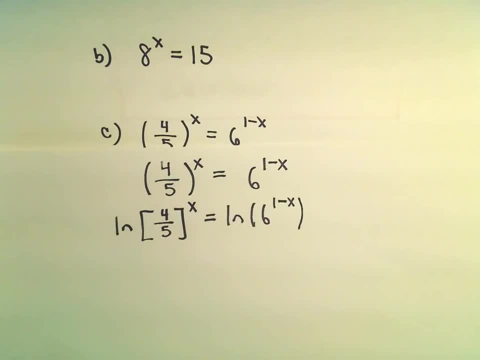 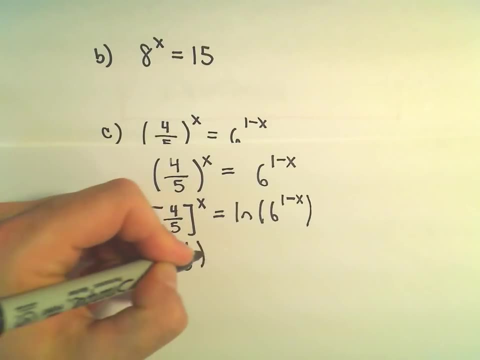 No particular reason I switched from brackets to parentheses. They're all the same to me. So the x would come out front on the left side and we'd have natural logarithm of 4 fifths On the right side, 1 minus x. 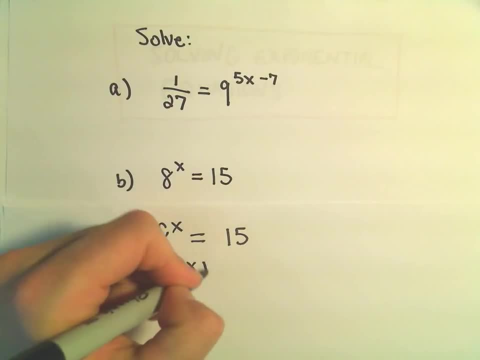 So I'm just going to take the natural logarithm of the left side. Well, hey, that means I have to take the natural logarithm of the right side as well. Okay, and don't get thrown off. You know the natural logarithm of 15, that's some number. 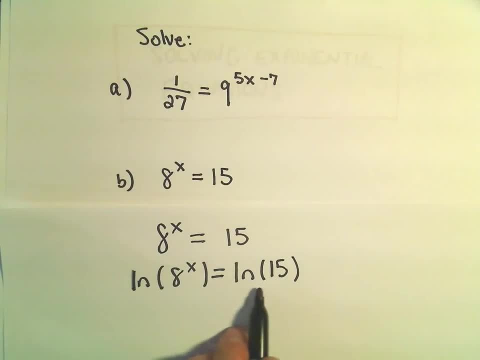 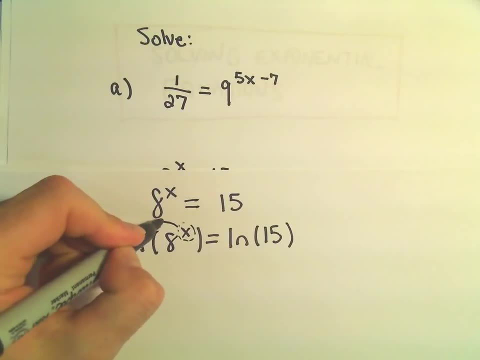 I always. you know I don't turn these into decimals because then you're approximating and I want to keep them exact. So remember this property that says: if you have exponents, you can bring them out front. And this is the whole point of using the logarithm in the first place. 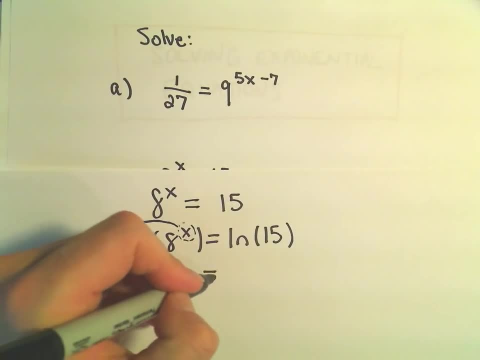 So on the left side we would have: x times the natural logarithm of 8 equals the natural logarithm of 15.. And well, if we want to solve for x, we can just simply divide both sides by that number, the natural logarithm of 8.. 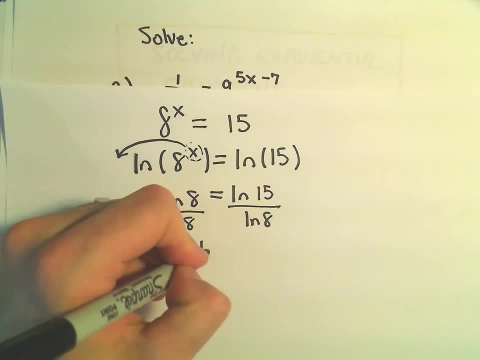 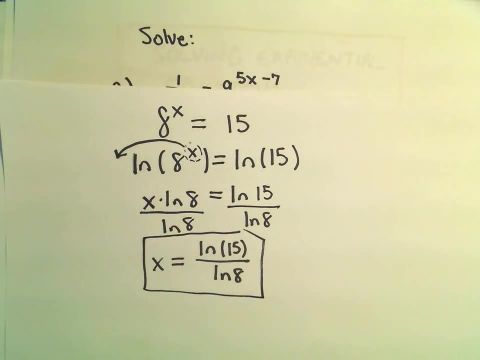 And on the right side we'll just have ln of 15 over ln of 8. And to me, hey, that's our solution. So again, you can always plug this into a calculator if you want a nice decimal approximation. 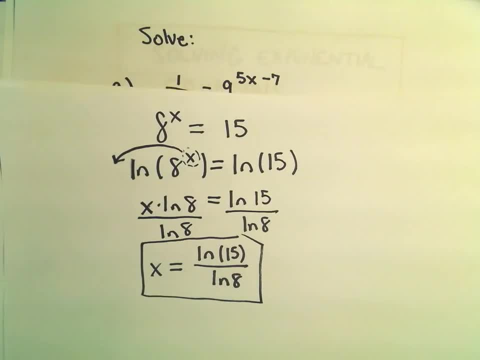 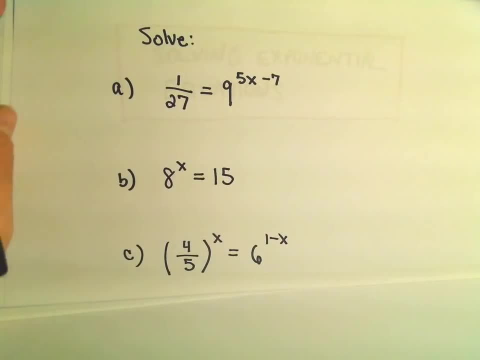 But You know, I'm just going to leave it right there. It's exact and hey, that's what we need. So one more example here We've got 4 fifths raised to the x equals 6 raised to the 1 minus x. 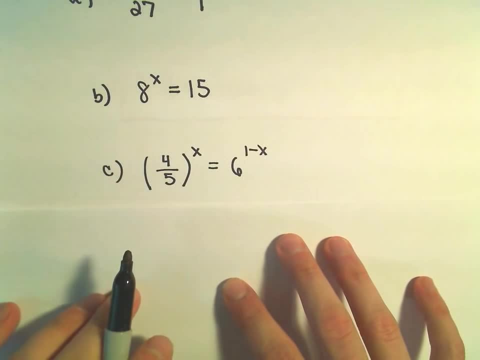 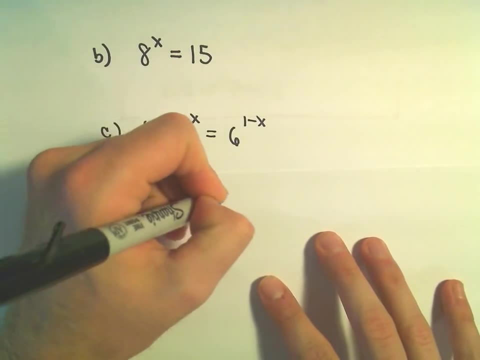 Well, exact same thing. You know, I see variables upstairs as exponents. The way I'm going to get those away from being exponents is by throwing logarithms onto both sides. Again, you can use any type of logarithm you want. 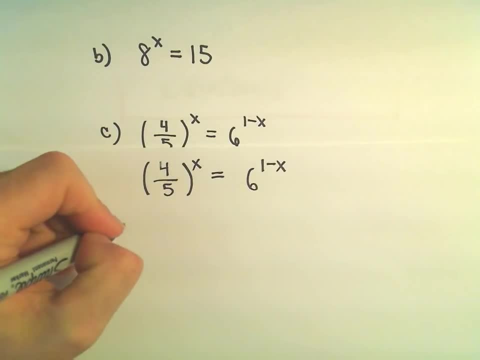 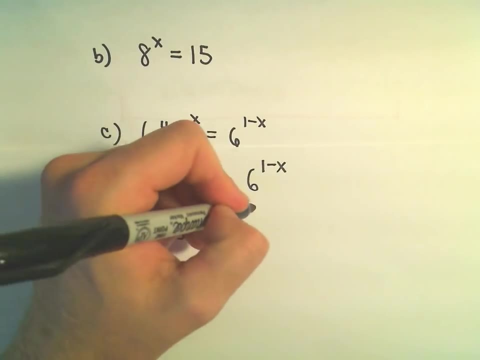 You obviously have to use the same one on each side. I'm just going to use the natural logarithm again. So we have: the natural logarithm of 4 fifths raised to the x equals the natural logarithm of 6 raised to the 1 minus x. 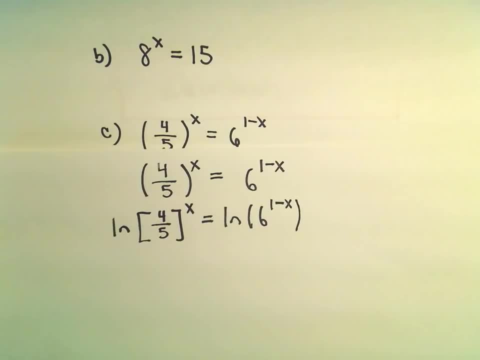 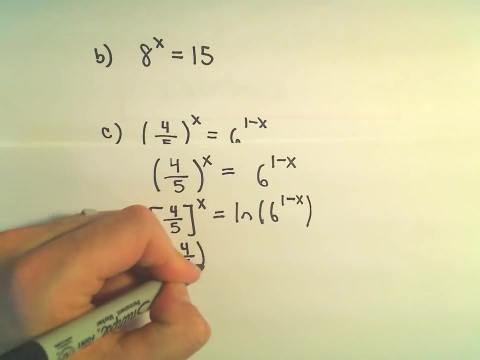 No particular reason I switched from brackets to parentheses. They're all the same to me. So the x would come out front on the left side and we'd have natural logarithm of 4 fifths On the right side. 1 minus x. that's our exponent. 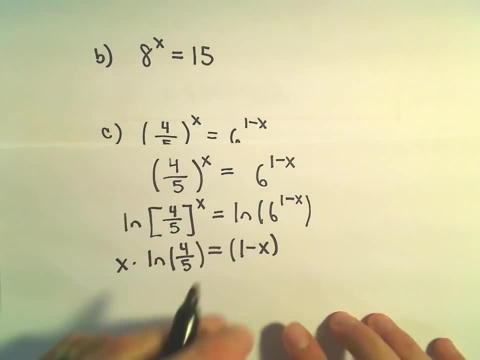 That's our exponent, so that's going to come out front Notice. I keep it in parentheses: times the natural logarithm of 6. And at this point this to me is just a linear equation. Again, don't be thrown off by the logarithm. 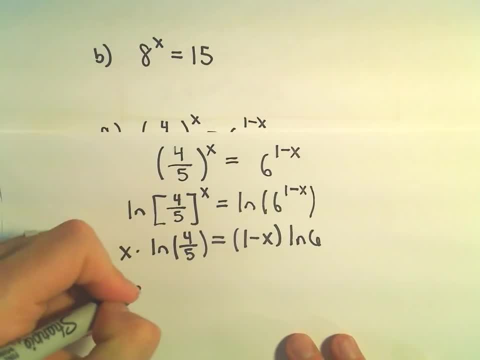 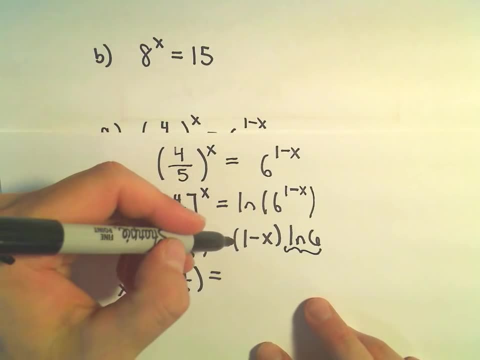 It's just a number. It's just a number. What I do is I get rid of all the parentheses. So on the right side, ln of 6, again is just a number. You could pretend it's sitting out front. 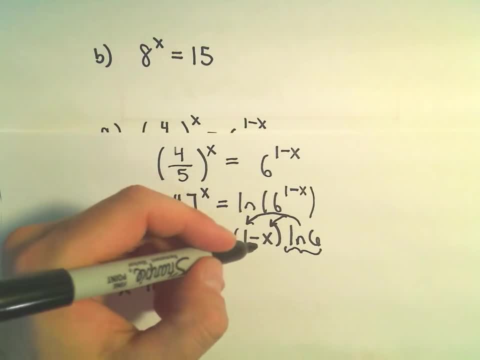 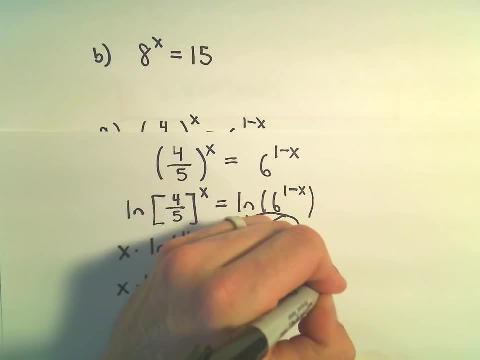 And in either case we have to distribute. We have to distribute it to both things, inside the parentheses. So ln of 6 times 1 is just ln of 6.. Then we'll get minus x times ln of 6.. And now what I'm going to do is I'm going to put my x's on the same side. 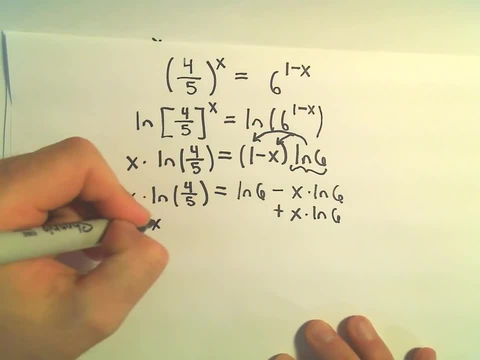 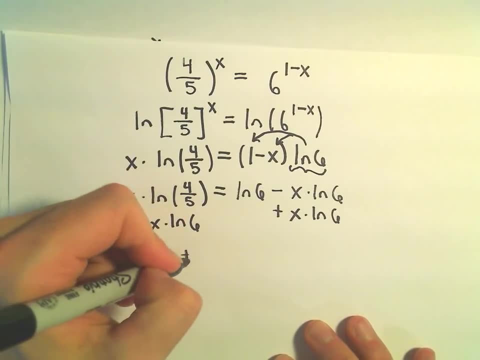 So I'm going to add x times ln of 6 to both sides. So on the left side we would have x times the natural logarithm of 4 fifths, plus x times the natural logarithm of 6.. On the right side, we would have x times the natural logarithm of 4 fifths. 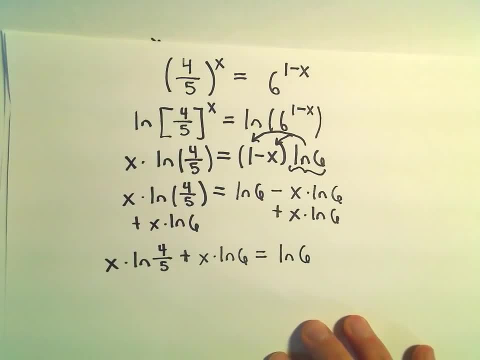 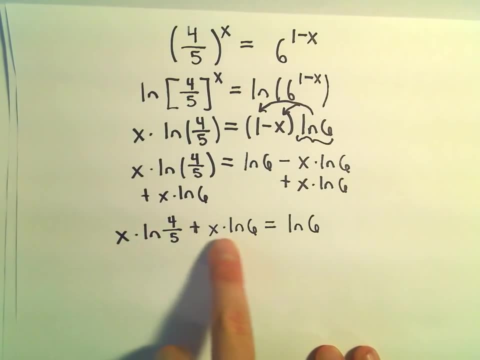 On the right side. we have just ln of 6 left over now And you know if this was a linear equation, you know well it is. But if we had nicer numbers, say 4 and 6, we would just add 4x and 6x. 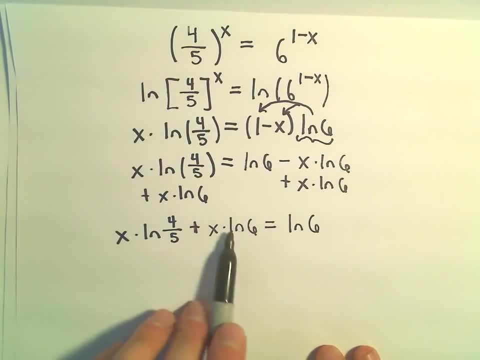 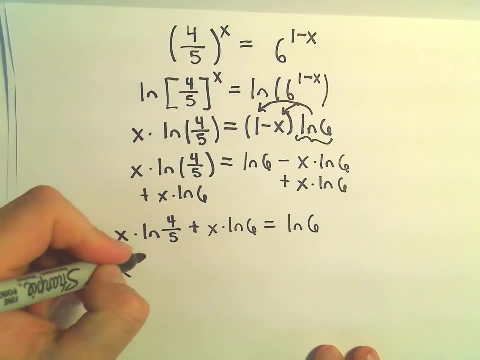 But you know, I don't know, ln of 4, fifths and ln of 6, I don't you know. well, I'm not too sure You could always put it in a calculator, But the idea is, algebraically you can just factor out the x. 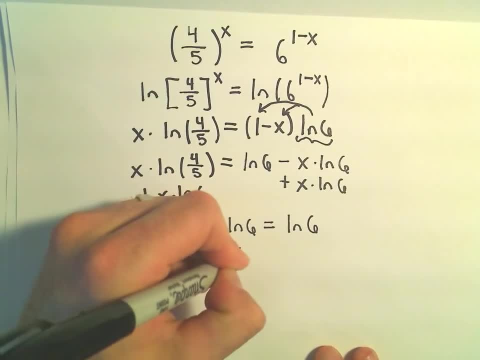 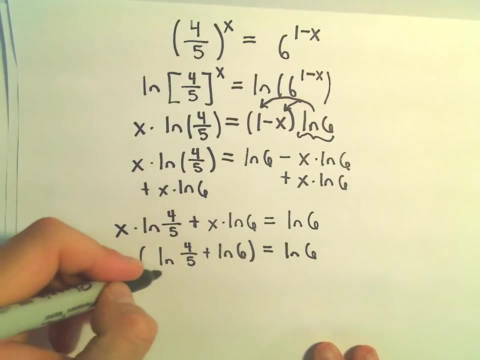 And then we have ln of 4 fifths plus ln of 6.. On the right side, we still have ln of 6.. And now, if we want to solve for x, we can simply divide both sides by this quantity: ln of 4 fifths plus ln of 6.. 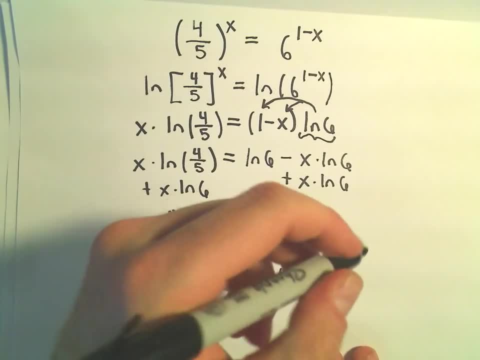 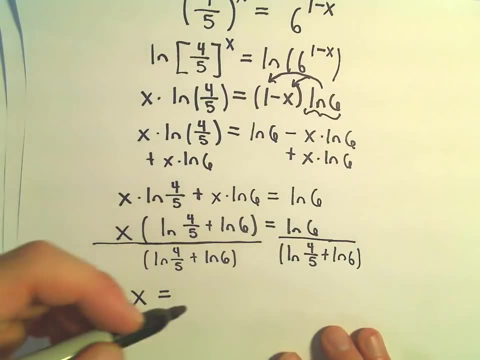 If I do it on the left, I've got to do it on the right. So ln of 4 fifths plus ln of 6. And on the left side we'll just be left with x, which is going to be what we want. 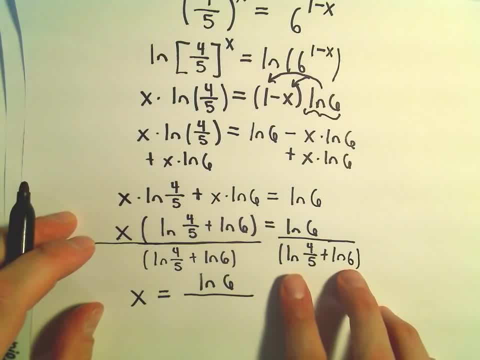 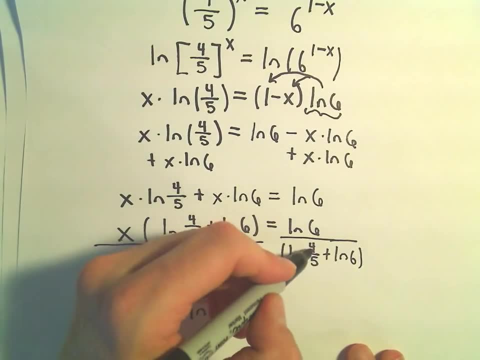 On the right side we have ln of 6. We could even combine our notice, our logarithm, in the denominator, because, right, we have addition and that means we can multiply. So we would take 4 fifths times 6, which would give us 24 fifths. 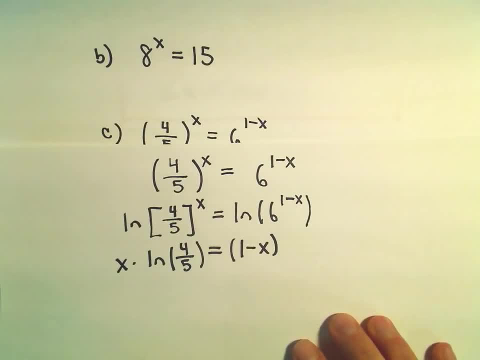 So that's going to come out front Notice- I keep it in parentheses- times the natural logarithm of 6. And at this point this to me is just a linear equation. Again, don't be thrown off by the logarithm. It's just a number. It's just a number. 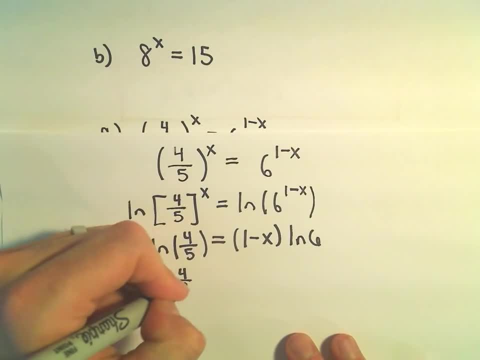 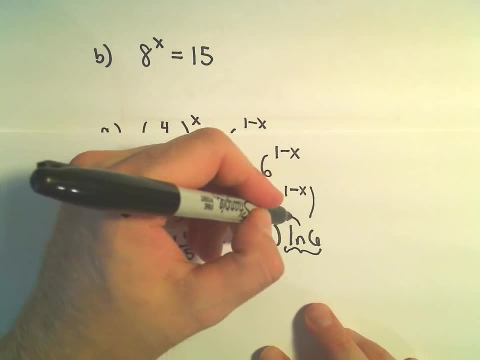 What I do is I get rid of all the parentheses. So on the right side, ln of 6 again is just a number. You could pretend it's sitting out front, And in either case we have to distribute it to both things inside the parentheses. 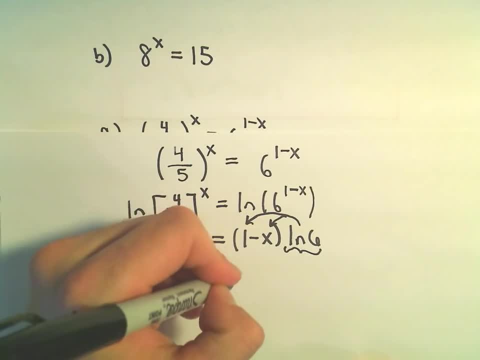 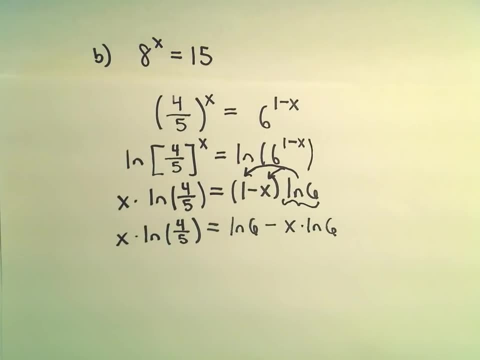 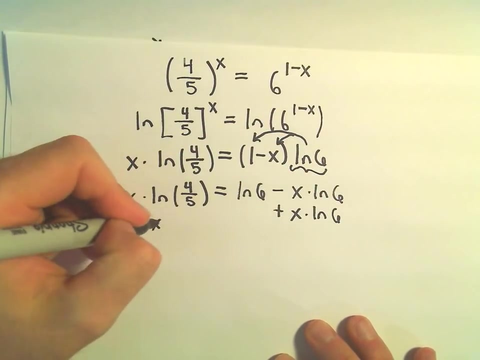 So ln of 6 times 1 is just ln of 6.. Then we'll get minus x times ln of 6.. And now what I'm going to do is I'm going to put my x's on the same side, So I'm going to add x times ln of 6 to both sides. 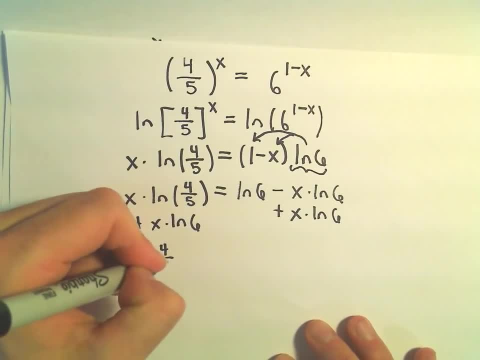 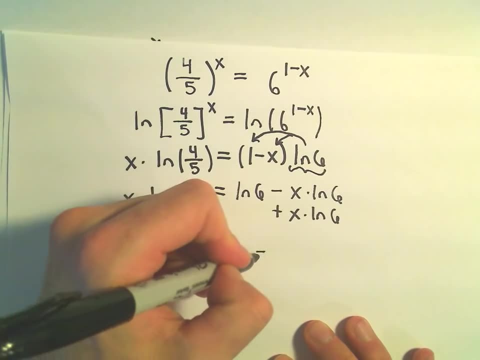 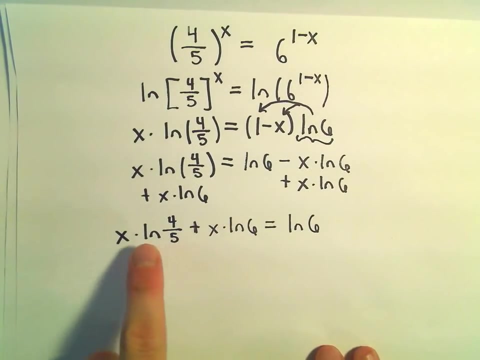 So on the left side we would have x times the natural logarithm of 4 fifths, plus x times the natural logarithm of 6.. On the right side, we have just ln of 6 left over now, And you know if this was a linear equation, you know well it is. 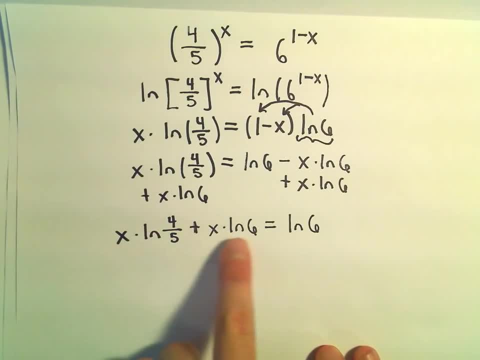 But if we had nicer numbers, say 4 and 6, we would just add 4x and 6x. But you know, I don't know, ln of 4 fifths and ln of 6, I don't you know. well, I'm not too sure. 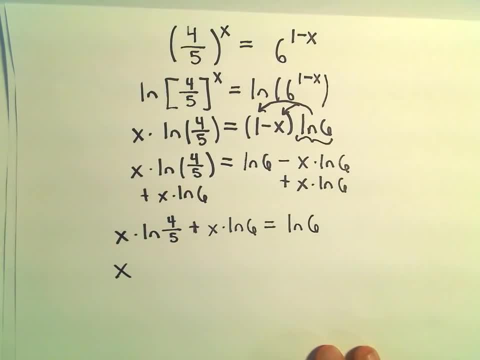 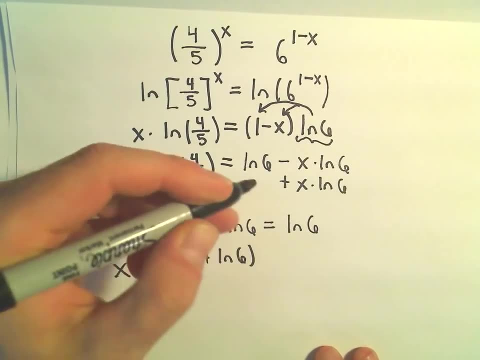 You could always put it in a calculator, But the idea is: algebraically you can just factor out the x And then we have ln of 4 fifths plus ln of 6.. On the right side we still have ln of 6.. 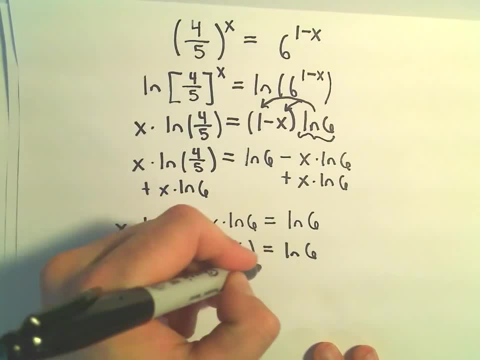 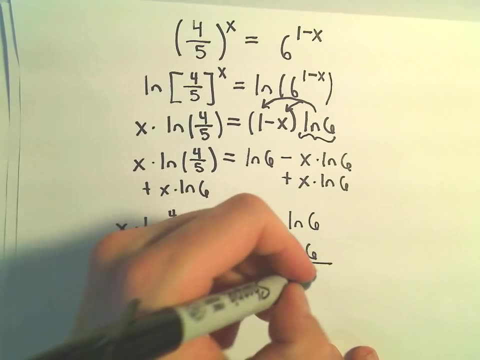 And now, if we want to solve for x, we can simply divide both sides by this quantity: ln of 4 fifths plus ln of 6.. If I do it on the left, I've got to do it on the right. So ln of 4 fifths plus ln of 6.. 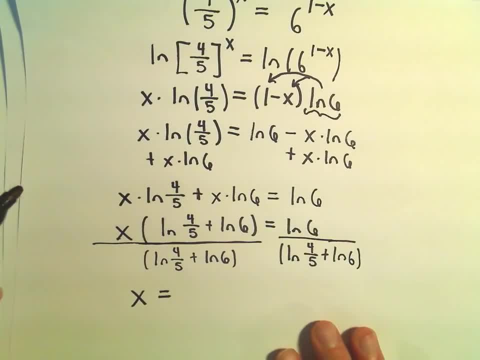 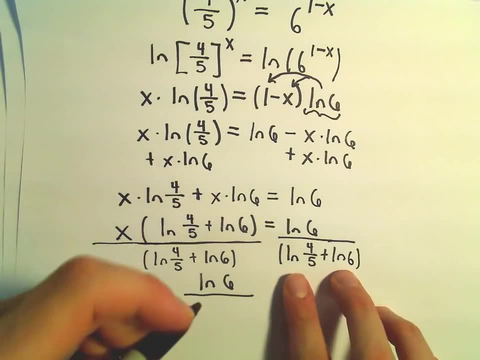 And on the left side, we'll just be left with x, which is going to be what we want. On the right side, we have ln of 6. We could even combine our… Notice our logarithm in the denominator, because, right, we have addition.